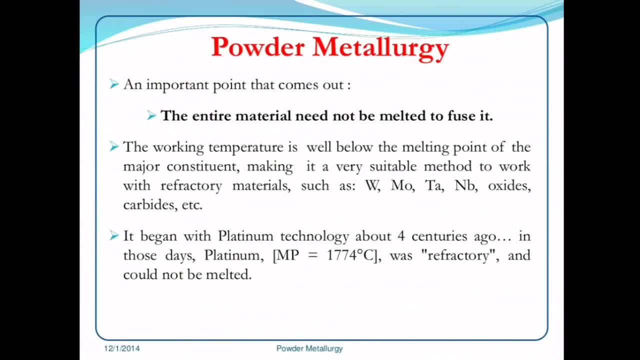 The entire material need not be melted to fuse it. The working temperature is well below the melting point of the major constituent. If the major constituent is the copper, then the working temperature is well below the melting point of the copper only. It is a very suitable method to work with refractory materials such as tungsten, molybdenum, tantalum, niobium, etc. 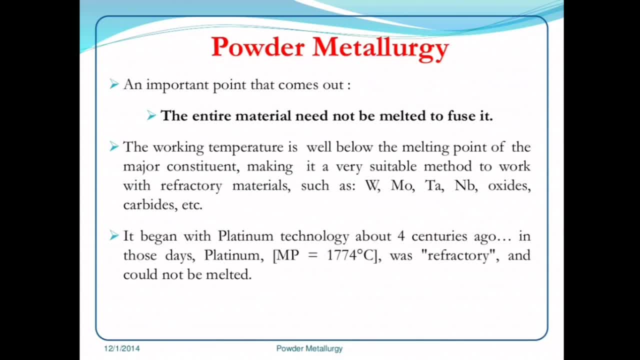 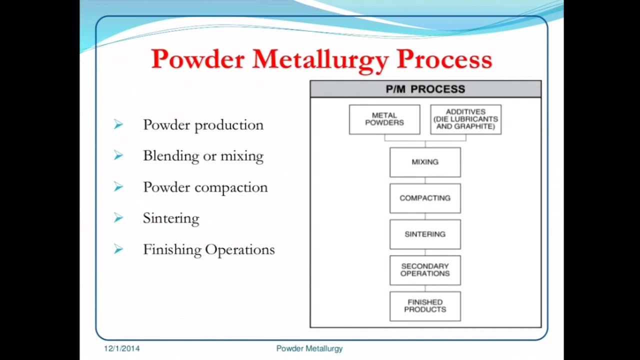 It began with platinum technology about four centuries ago. In those days, platinum of melting point 1774°C was refractory and could not be melted. Powder metallurgy process. There are five processes: Powder production, Blending or mixing, Powder compaction, Sintering. 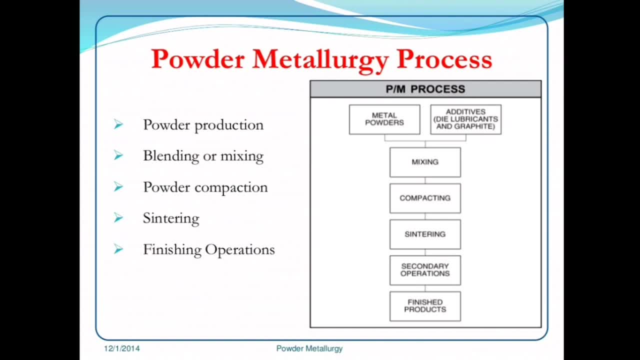 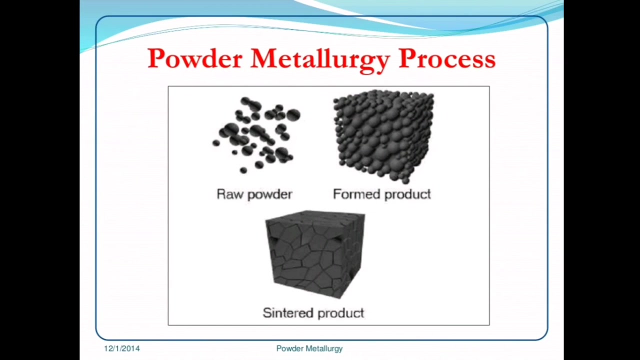 Finishing operation. The schematic diagram shows the powder metallurgy process. Metal powders and additives such as dilubricants and graphite are mixed together. Compacting, Sintering. Sintering means heating, Secondary operations and finished products. This is the powder metallurgy process diagram shows a raw powder. 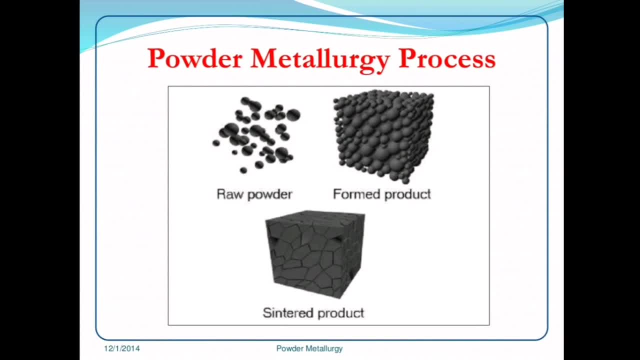 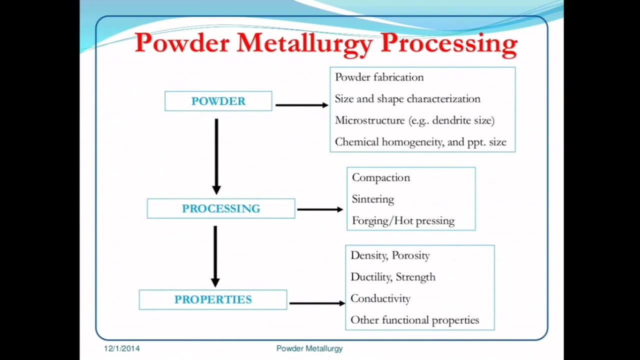 Which is compacted, that is, a formed product, and then sintered to make a solid block of the metal Powder metallurgy process. The steps includes powder fabrication, size and shape, characterization, microstructure example, dendritic size, chemical homogeneity and precipitate size. 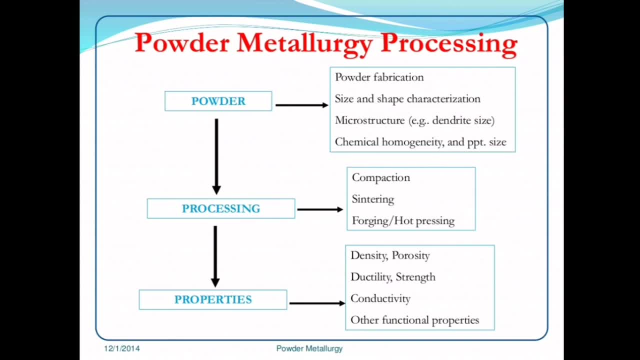 Processing, Compaction, Sintering, Forging or hot pressing Properties: Density, Porosity, Ductility, Strength, Conductivity And other functional properties. Usual powder metallurgy production sequence: Blending and mixing With help of rotating drums, blade and screw mixers As shown in the diagram. 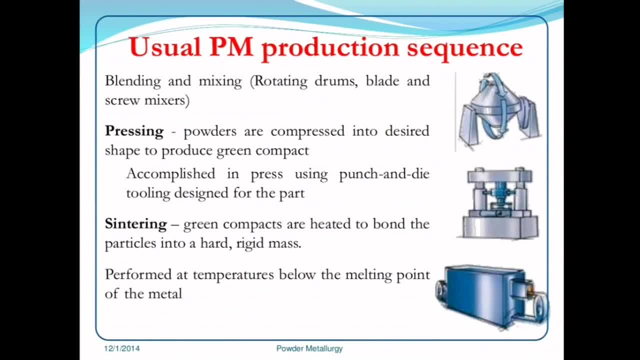 Then pressing powders or hot presses. This is the process: Powder production, Sintering, Forging or hot pressing. Properties: Density, Porosity, Ductility, Strength, Conductivity And other functional properties. Usual powder metallurgy production sequence. Blending and mixing Powders are compressed into desired shape to produce green compact. 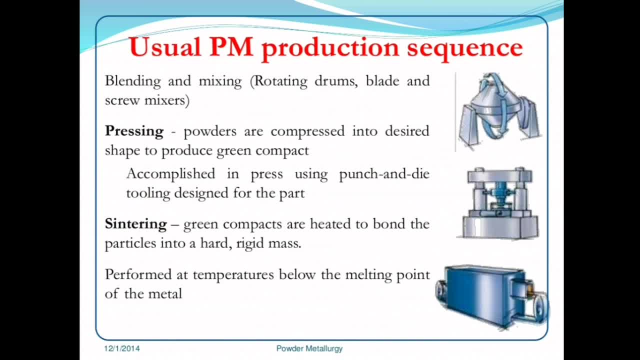 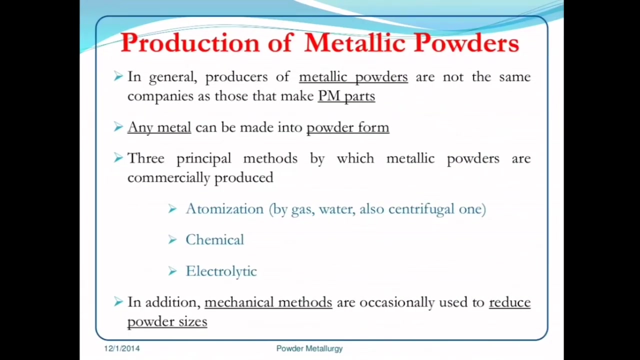 Accomplished in press using punch and die tooling designed for the part Sintering. Green compacts are heated to bond the particles into the hard, rigid mass, Performed at temperature Just below the melting point of the metal. In general, producers of metallic powders are not the same of the companies as those 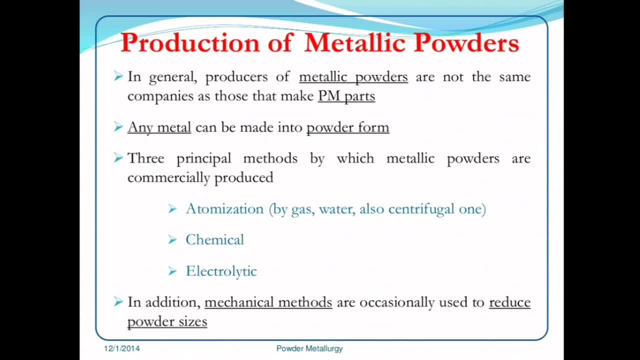 that make powder metallurgy parts. Any metal can be made into powder form. Three principal methods by which metallic powders are commercially produced are Automization By gas, Water, Also centrifugal one, Chemical And electrolytic. In addition, mechanical methods are occasionally used to reduce the powder sizes. 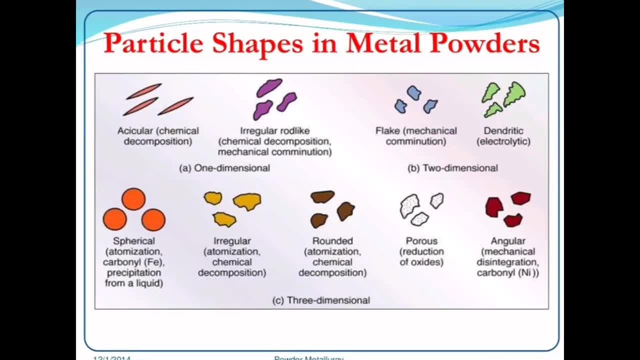 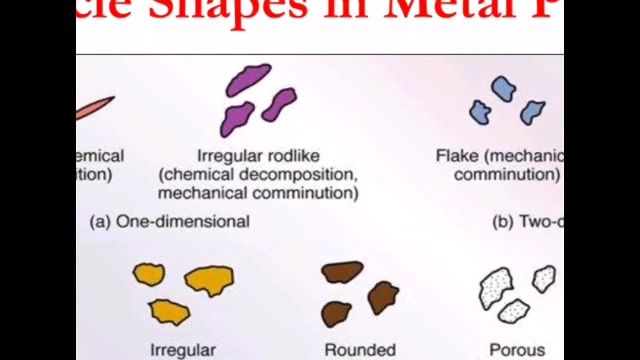 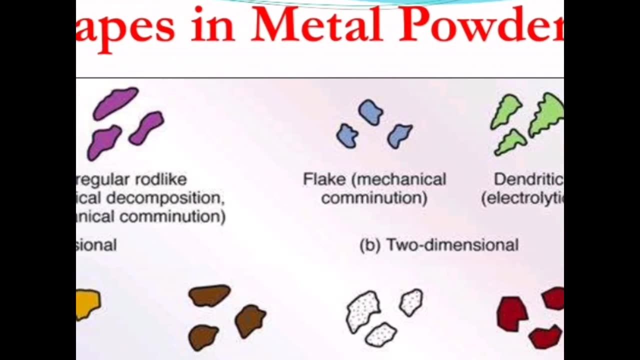 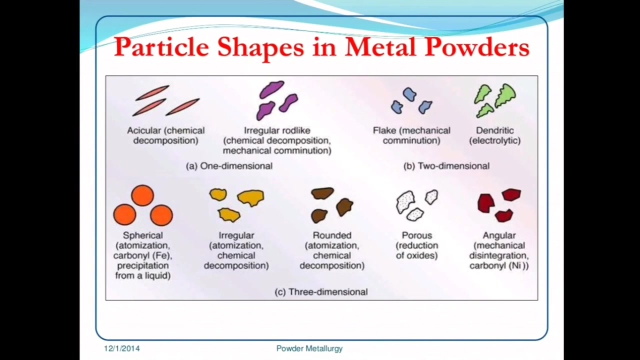 These are the powder sizes, The particle shapes in metal powders: A-Circular Chemical decomposition: Irregular Rod-like Chemical decomposition. Mechanical combination, Flake, Mechanical combination, Dendritic, Then Sperical Automization. Carbon and iron Residuation from the liquid. Irregular Automization. 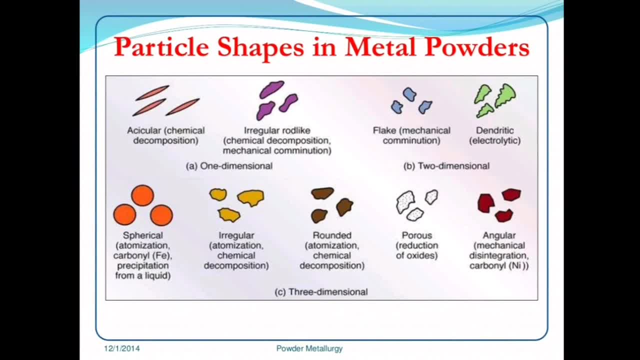 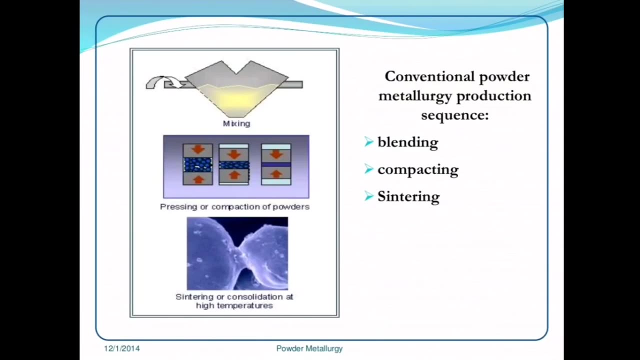 Chemical decomposition: Rounded Automization. Chemical recomposition, Porous reduction of oxides, Angular Mechanical disintegration. Carbon in Ni, Conventional Powder. metallurgy: production sequence: Blending, Compacting, Sintering, Sintering, Sintering, Sintering, Sintering, Sintering, Sintering. 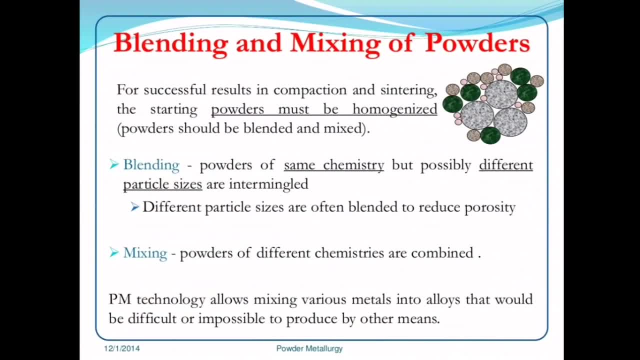 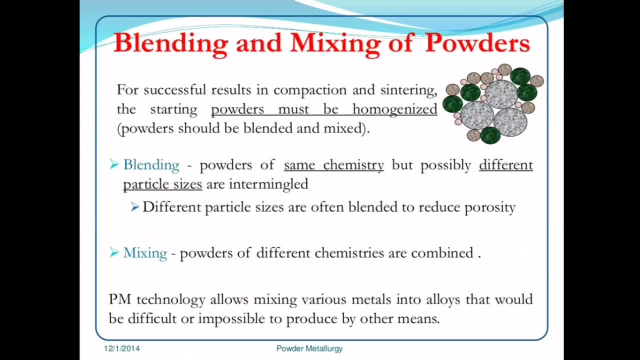 Blending and Mixing of Powder Powders. For successful results in compaction and sintering, the starting powders must be homogenized, That is, the powder should be blended and mixed with same materials. Blending Powders of same chemistry but possibly different particle sizes are intermingled. 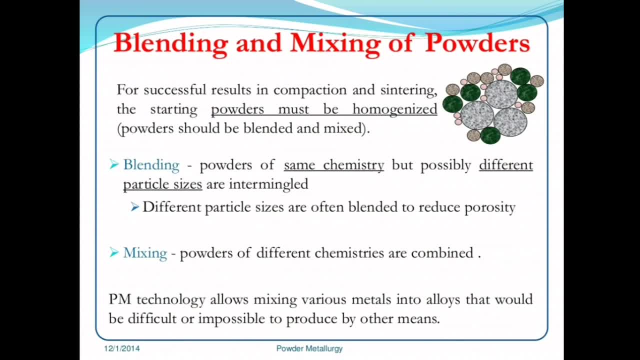 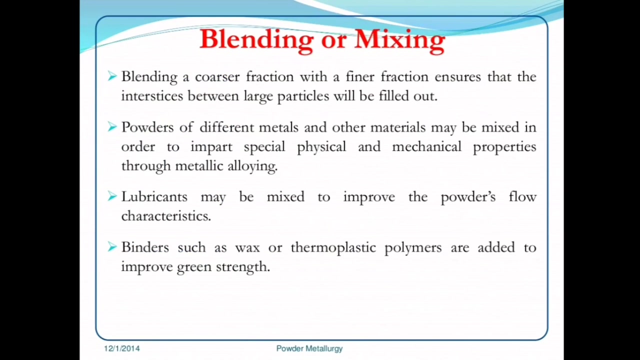 Different particle sizes are often blended to reduce the porosity. Mixing Mixing powders of different chemistries are combined. Powder metallurgy technique allows mixing various metals into alloys that would be difficult or impossible to produce by other methods. Blending a coarse fraction with a finer fraction ensures that the interstice between large particles will be filled out. 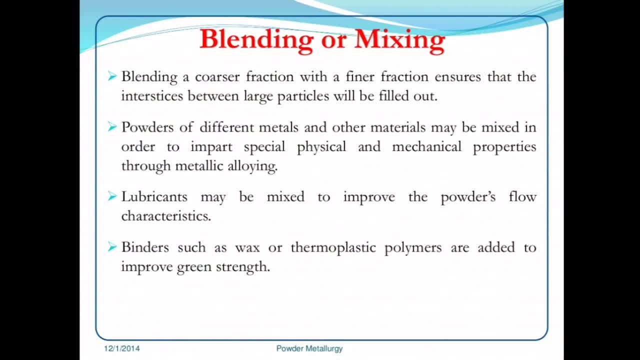 Powders of different metals and other materials may be mixed in order to impart special physical and mechanical properties through metallic alloying. Lubricants may be mixed to improve the powder's flow characteristics. Binders such as wax or thermoplastic polymers are added to improve grain strength. 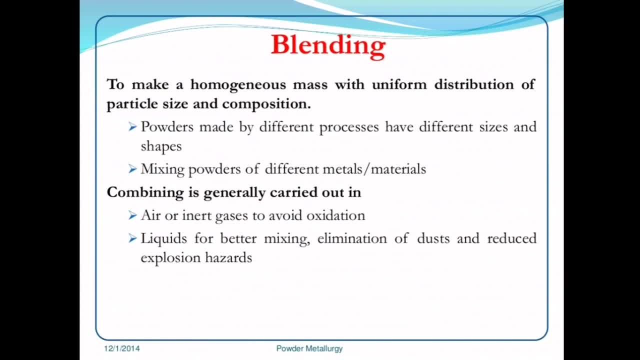 To make a homogeneous mass with uniform distribution of particle size. powders made by different processes have different sizes and shapes. Mixing powders of different metals or materials when combining is generally carried out in air or inert gases to avoid oxidation. Liquids for better mixing, elimination of dust and reduced explosion hazards. 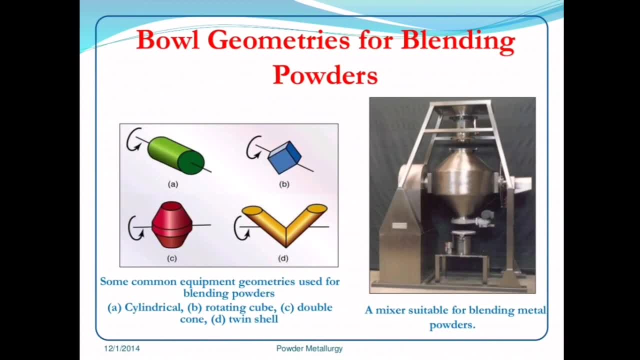 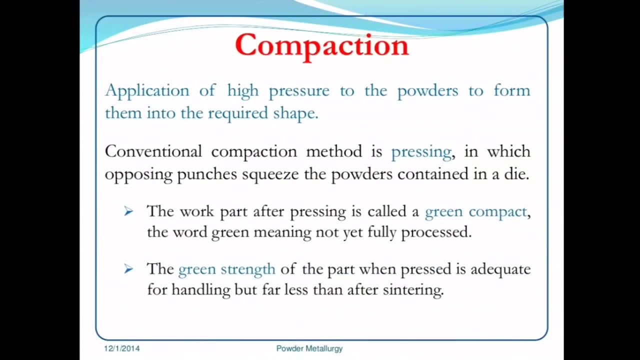 The diagram shows the bowl geometries for blending powders. Compaction: Application of high pressure to the powders to form them into the required shape. Conventional compaction method is pressing using hydraulic press, in which the opposing punches squeeze the powders contained in a die. 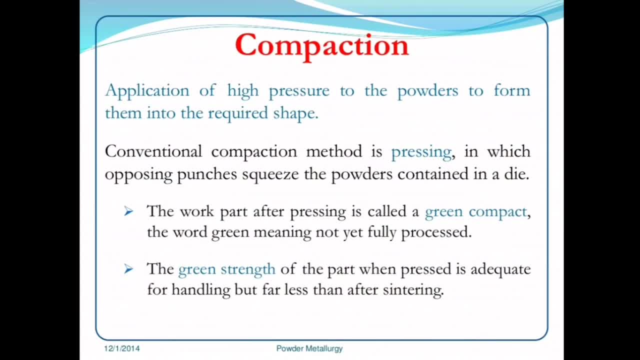 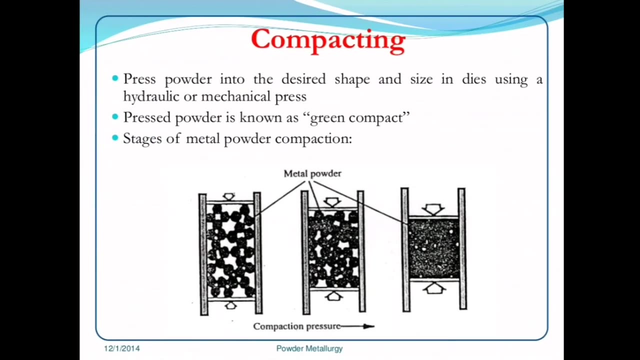 The work part after pressing is called as the green compact. The word green means not yet fully processed. The green strength of the part when pressed is adequate for handling, but far less than after stinting. Compacting Press powder into the desired shape and size in the dies using a hydraulic or mechanical press. 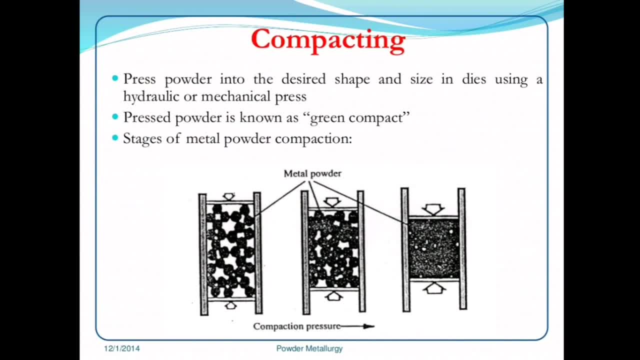 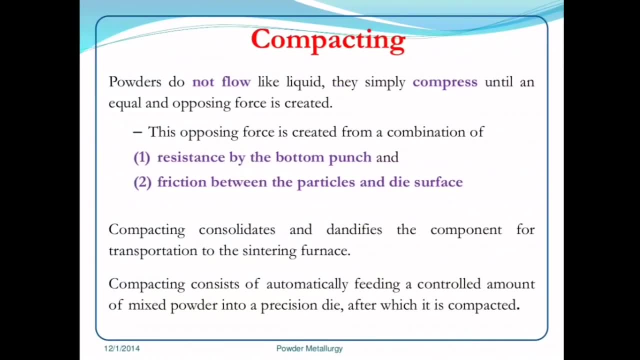 Press, the powder is known as green compact. Stages of metal production metal powder compaction are shown below: Compacting: Compacting Powders do not flow like liquid. They simply compress until an equal and opposing force is created. This opposing force is created from a combination of the resistance by the bottom punch and friction between the particles and die surface. 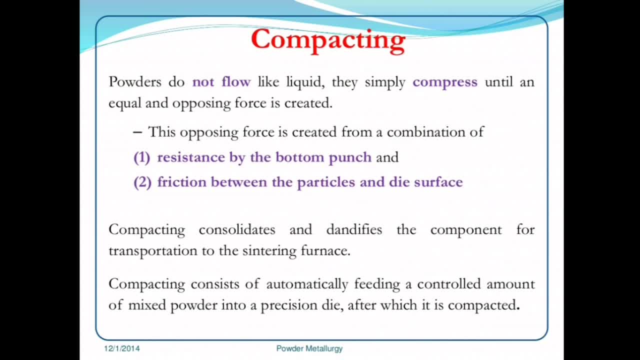 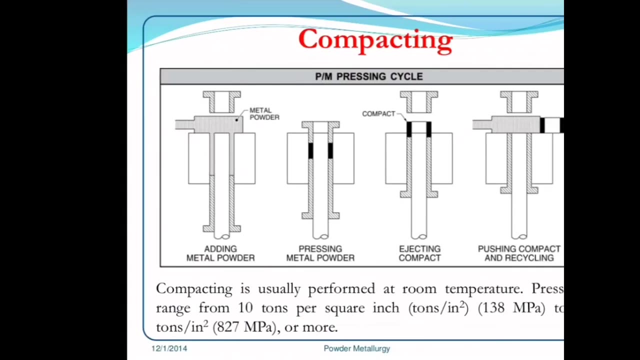 Compacting consolidates and dandifies the components for transportation to the sintering furnace. Compacting consists of automatically feeding a controlled amount of mixed powder into a precision die, after which it is compacted. Compacting, Compacting, Compacting, Compacting, Compacting. 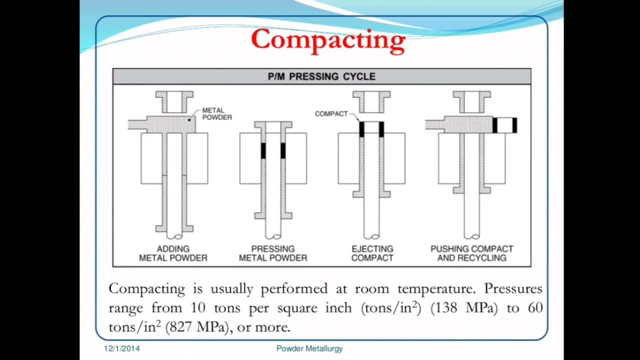 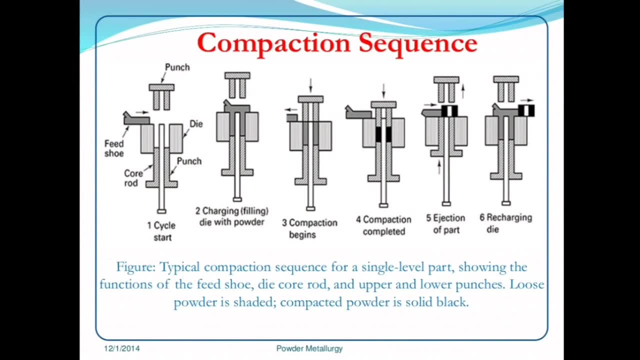 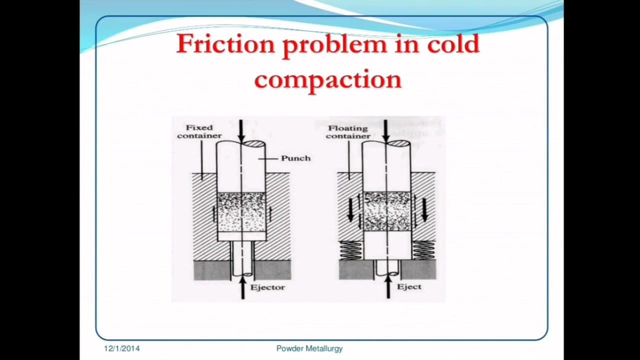 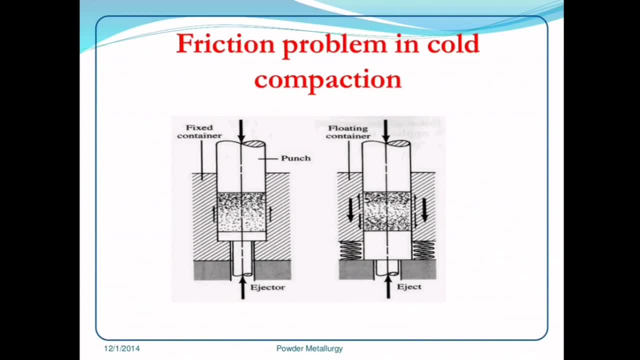 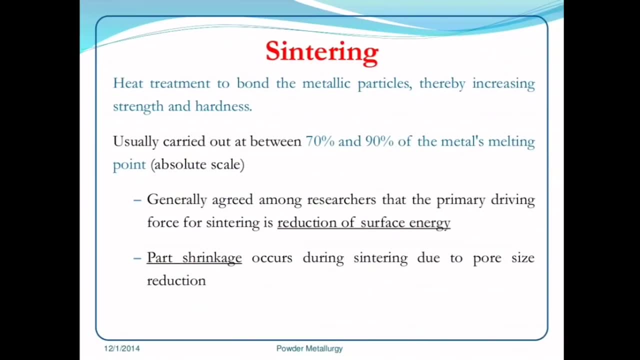 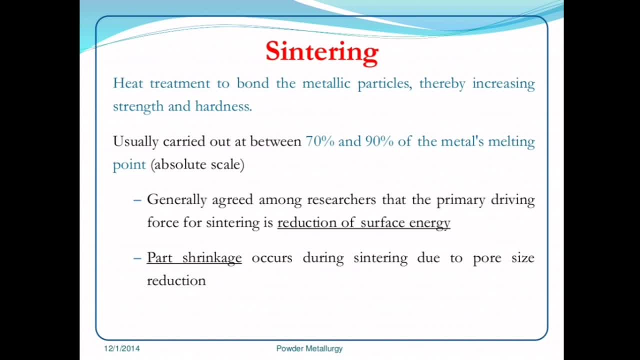 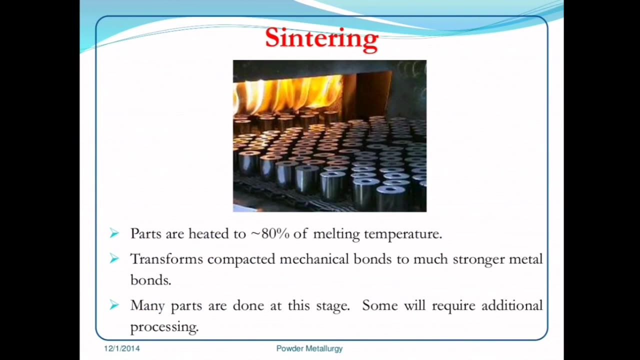 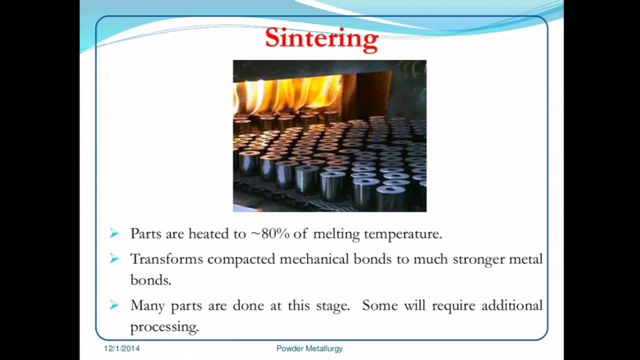 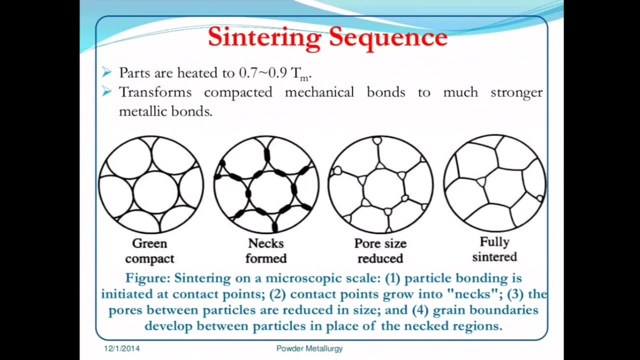 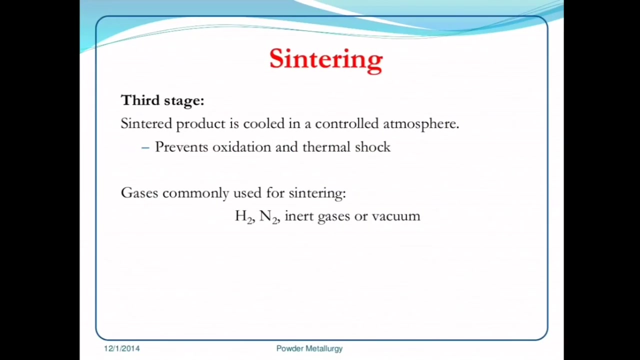 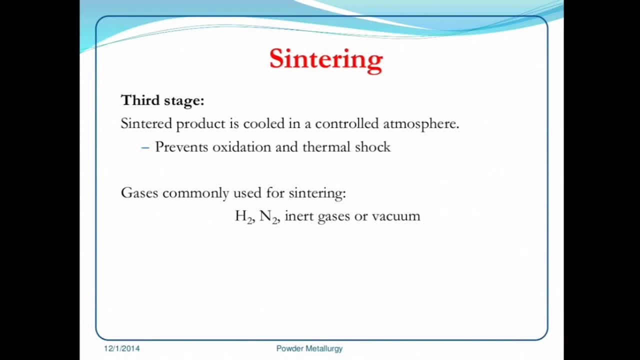 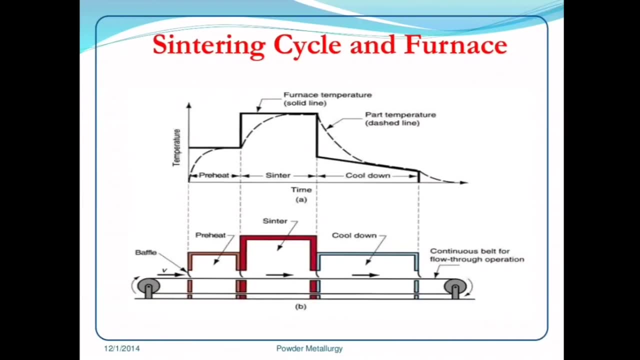 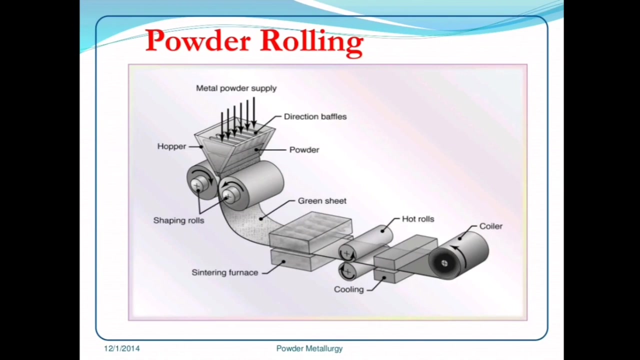 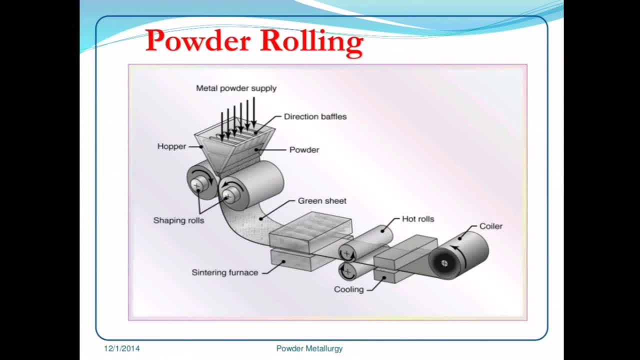 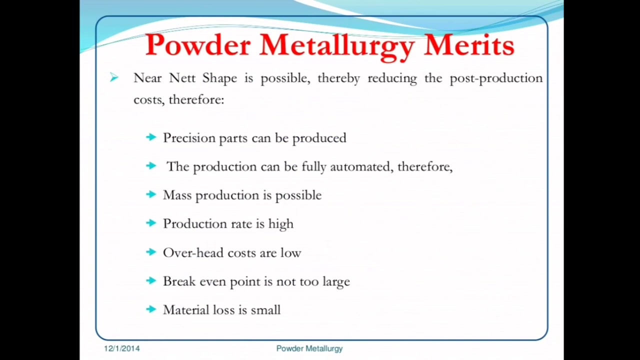 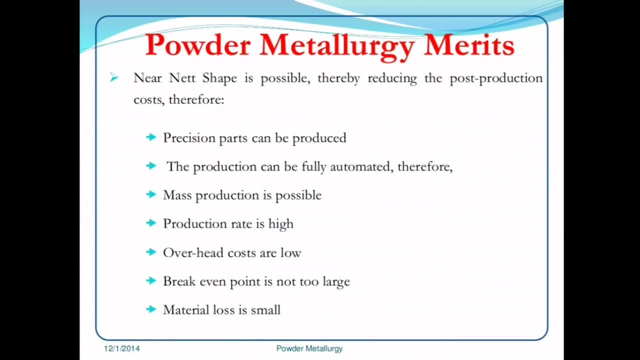 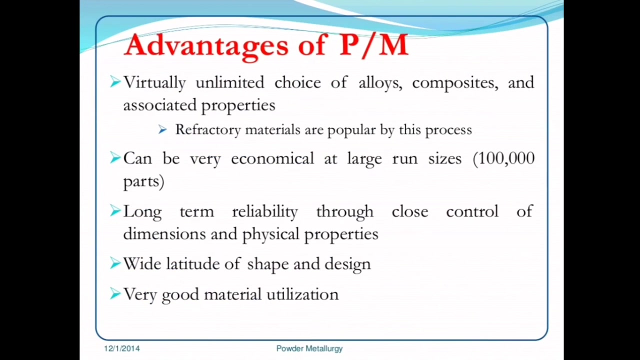 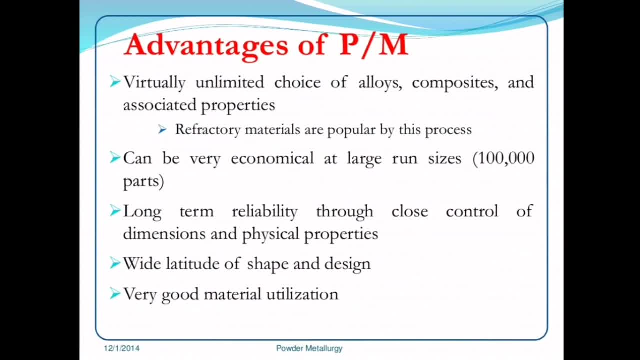 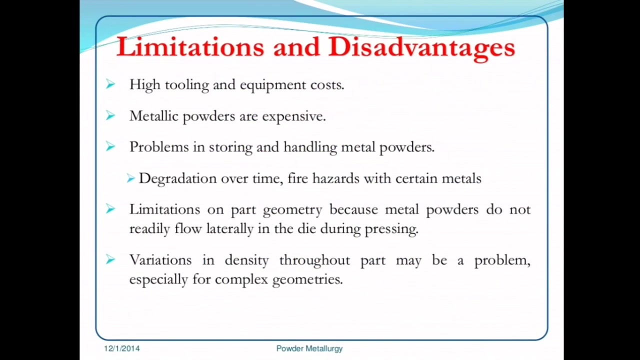 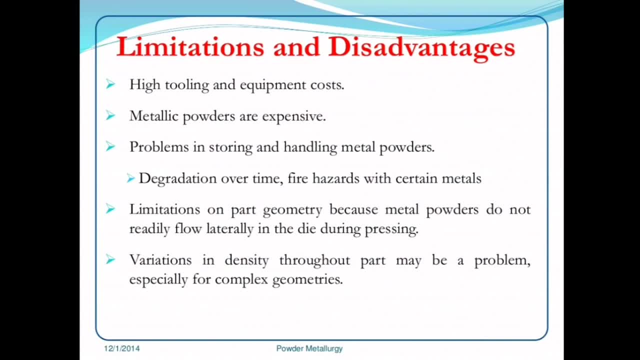 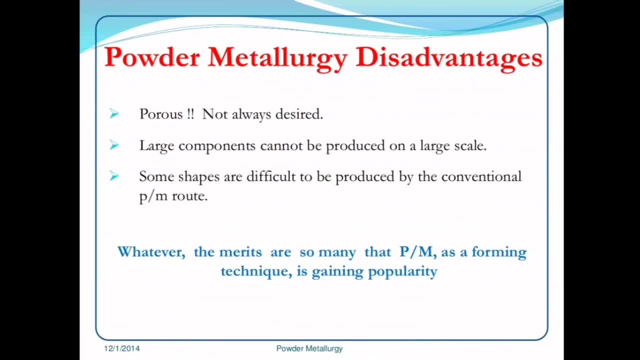 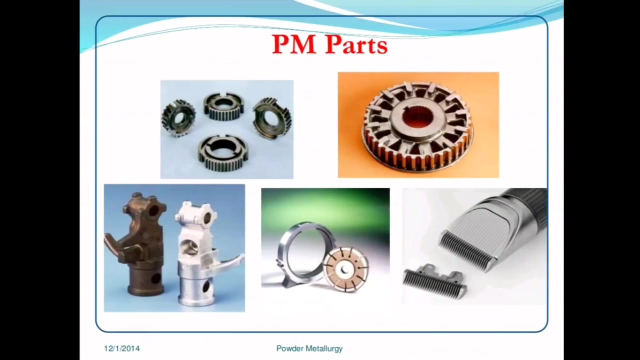